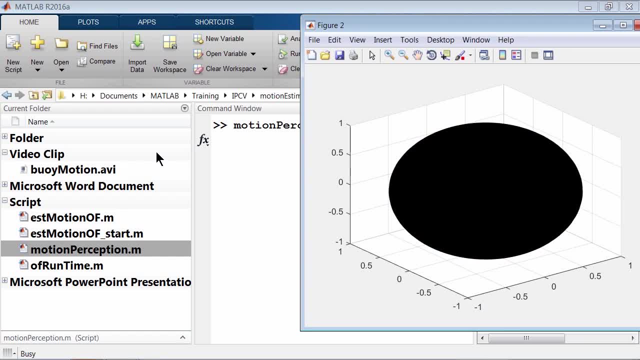 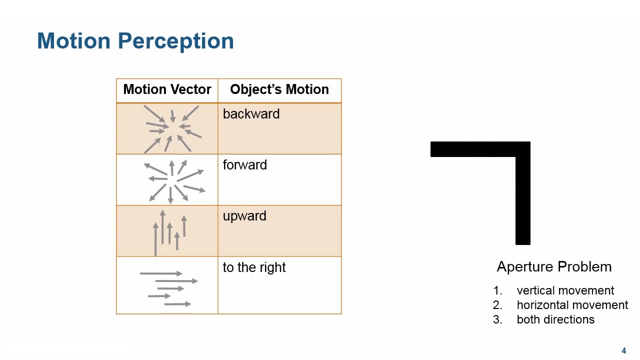 If we look at a rotating uniquely colored sphere, we will recognize movement. however, if we look at a rotating uniformly colored sphere, we will not recognize any movement. Let's go back to the presentation. Motion estimation methods return motion vectors and it is important to interpret them correctly. 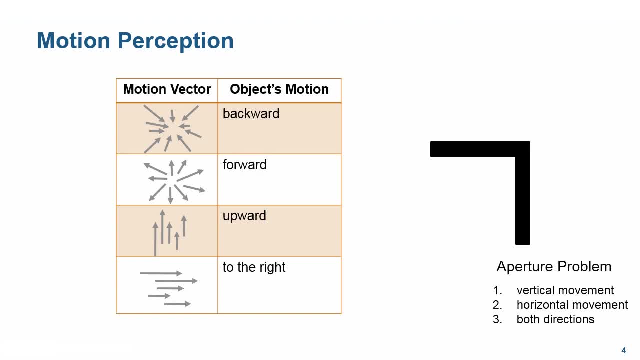 We see them in this table. Arrows going inwards mean the motion is backward. Arrows going outward means the motion is forward. Apart from this, arrows to the left, right, top and bottom refer to likewise motions. One way to compute the motion vectors is to use the optical flow technique. 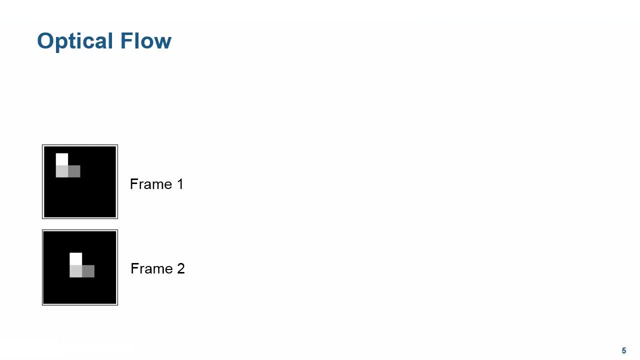 Given a sequence of grayscale images, we assume that the intensity structures of an object are constant over time, at least between immediate frames. Here we have two frames where the object has moved in frame 2. This is called gray value constancy assumption. 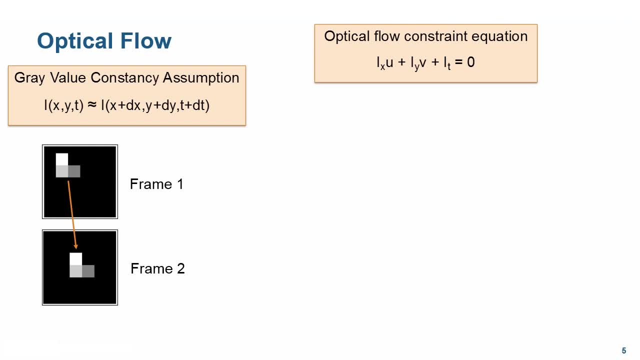 This results in the optical flow constraint equation. as can be seen here In this equation Ix, Iy and It are image gradients. Image gradients are used to compute the directional change in intensity or color. Ix and Iy are spatial brightness gradients of frame 1.. 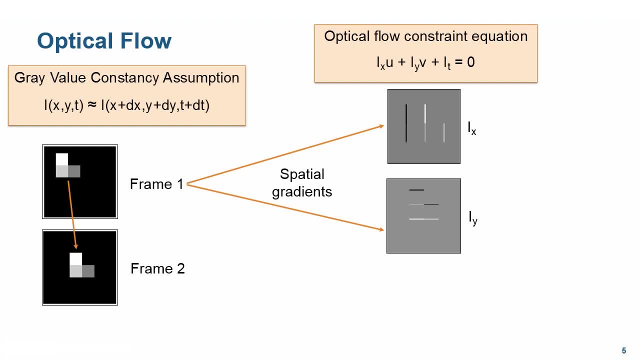 Ix shows the vertical edges in the image and Iy shows the horizontal edges in the image. It is the temporal brightness derivative between frames 1 and 2.. Both the spatial and temporal gradients are obtained using different types of image filters. The filters used vary with respect to each of the optical flow method. 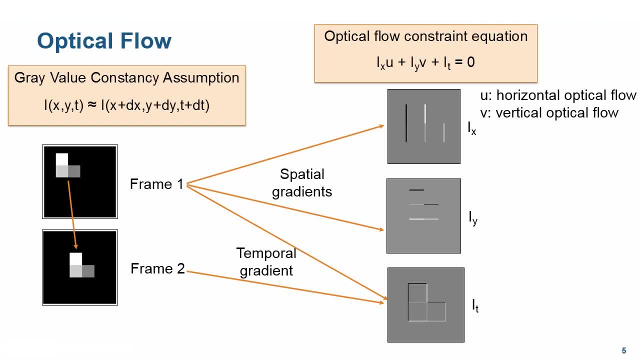 U and V in the equation are the flow vectors that we are ultimately using. What are we going to be interested in? The formula states that if we apply the flow vectors to the spatial gradients of an image, it will be canceled by the temporal gradient. 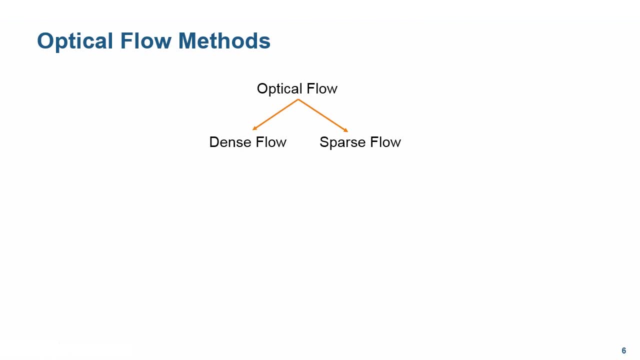 As we saw in the introduction, there are several optical flow methods available. These can be broadly classified into dense flow and sparse flow techniques. In dense flow methods, we process the entire image and hence all the pixels. In sparse flow methods, we process only a part of the image or a subset of pixels. 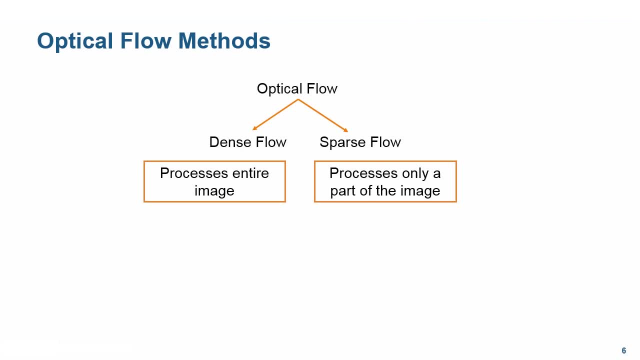 Consequently, the dense flow methods tend to be more accurate but could be computationally intensive. Sparse flow methods could be computationally fast but could be less accurate. The horned, shrunk and farmed back methods are dense flow methods. Lucas-Canade is a sparse flow method. 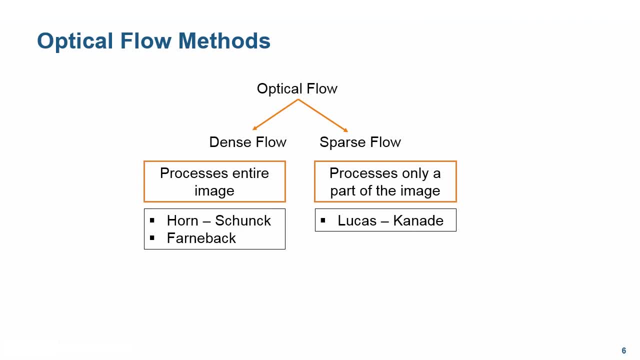 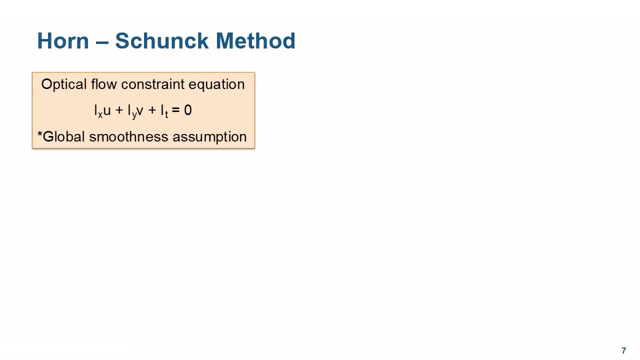 Please note that, regardless of the type of optical flow methods used, all these algorithms use intensity images to estimate motion. Let's first take a look at the horned shrunk method and see how to perform optical flow. This method attempts to solve the general optical flow constraint equation for the motion. 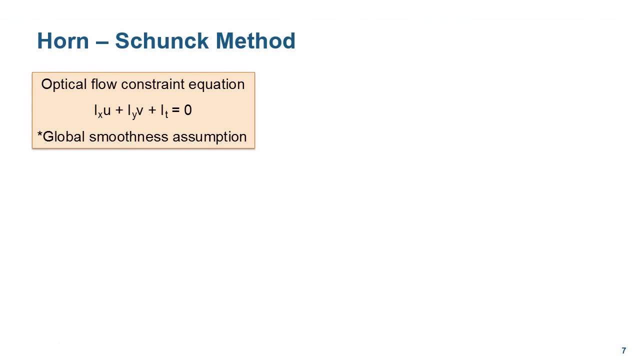 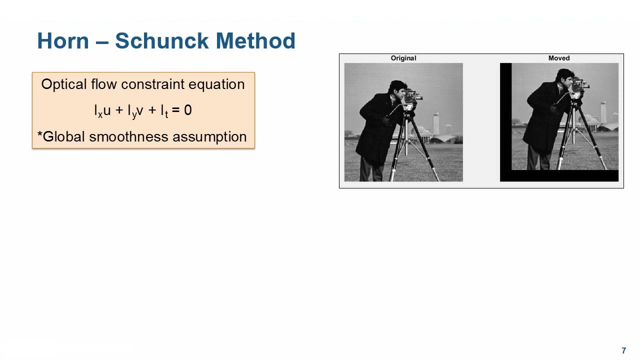 vectors u and v. Apart from the already stated optical flow problem, the method has an extra global smoothness assumption According to which all the pixels between consecutive frames move similarly If we have two image frames. the horned shrunk method uses a Sobel filter to calculate the 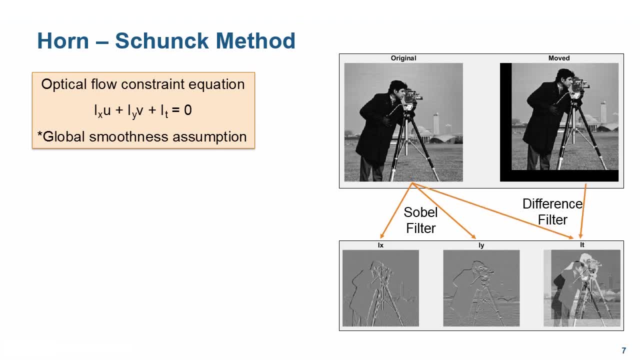 spatial gradients and a difference filter to calculate the temporal gradient. After this, the method iteratively solves for u and v, our optical flow vectors. We can apply this using the optical flow object. Then we call estimateFlow on the object, with the image as an argument to estimate the optical. 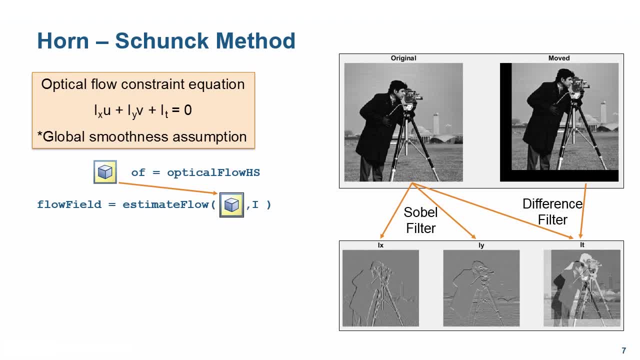 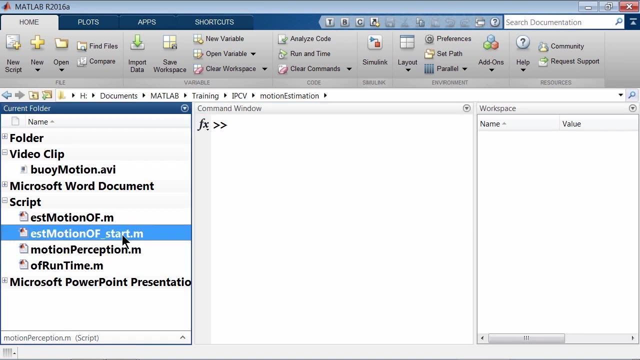 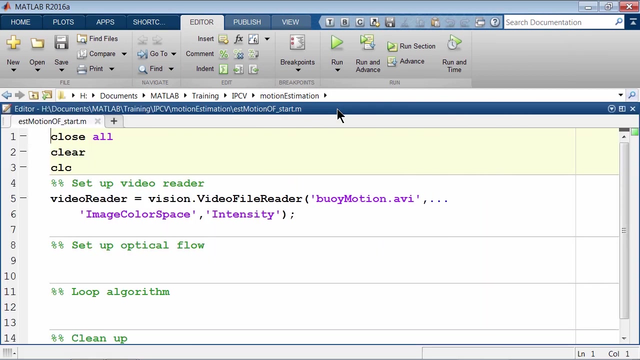 flow. The resulting flow field is also an object that stores the direction and speed of one VideoFrame to another. Let's switch to MATLAB to see how we can use this. Open the starter script: estimateMotionOpticalFlow- underscore- start. In this script we have already been provided with starter code. 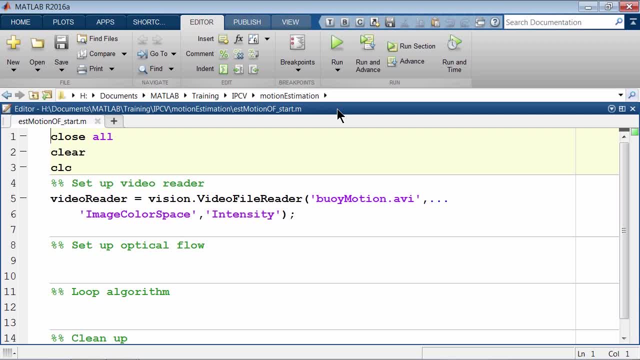 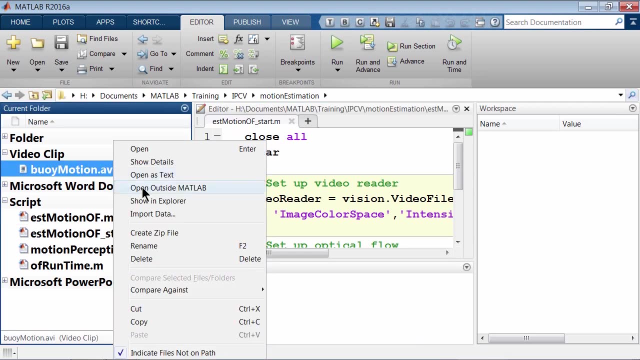 and comments that will help us develop our algorithm. We see the video file reader system object that has been set up to read the file buimotionavi. We can take a look at this file in the current folder here. Right-click on this file and open it outside MATLAB. 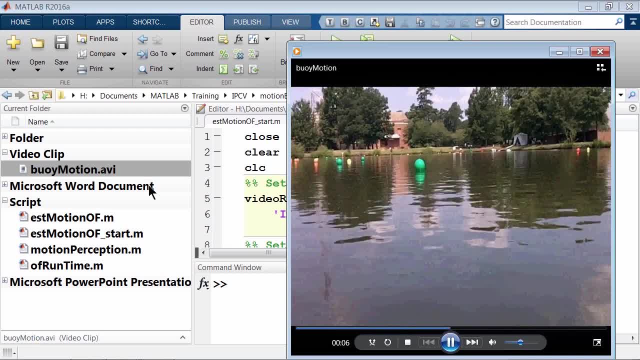 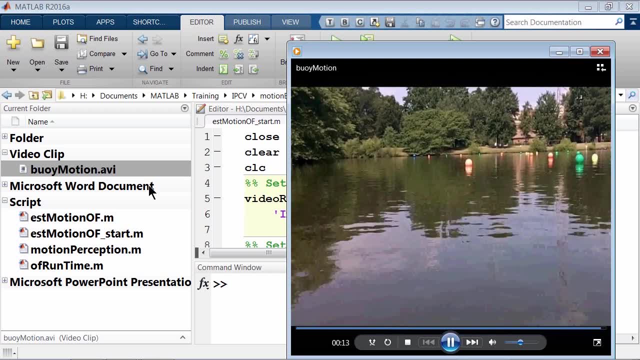 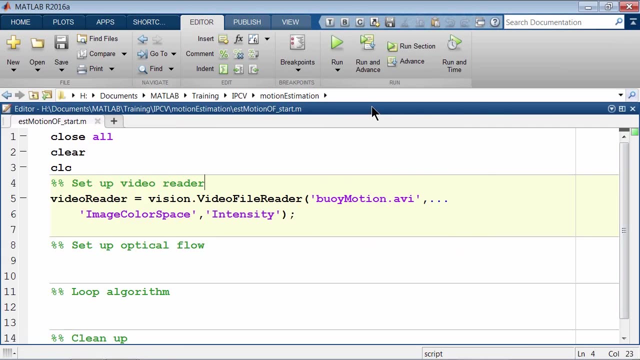 This is the video we will be analyzing to detect if the robot boat is moving towards the right or left. Let's go back to the script. Note that we are reading the video frames as an intensity frame. Now let's set up the optical flow. 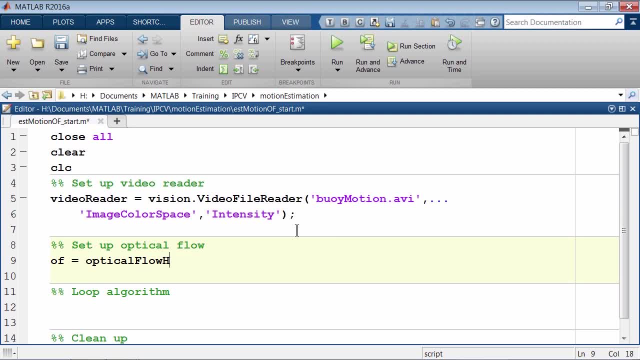 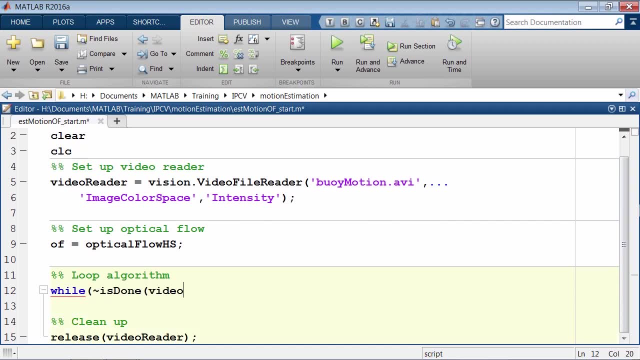 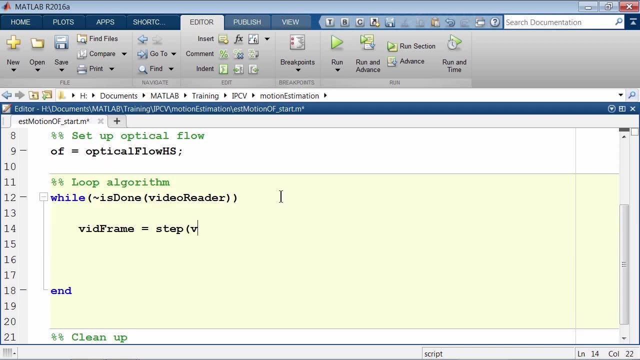 To use the Horn-Schrank method. we will use optical flow HS object. This is the first step To apply this on our video frames. let's use a while loop as before. We will read in a video frame Then to obtain the optical flow field. 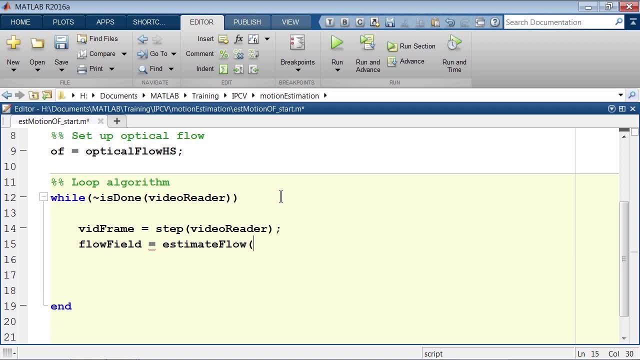 we will use the estimate flow function on the optical flow HS object with the current frame or the image as an argument. Flow field is an optical flow object that stores the direction and speed of all the pixels of the current frame with respect to the previous frame. 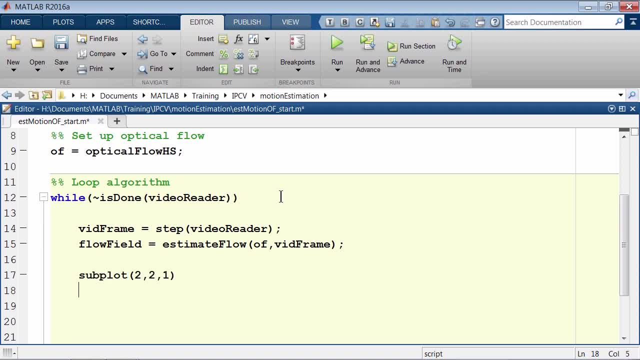 We can now visualize the result of the optical flow using the plot command, which automatically takes in this object as an input. For this particular type of input, we can specify additional properties to the plot command to control the visualization Decimation factor, controls the downsampling of the vectors. 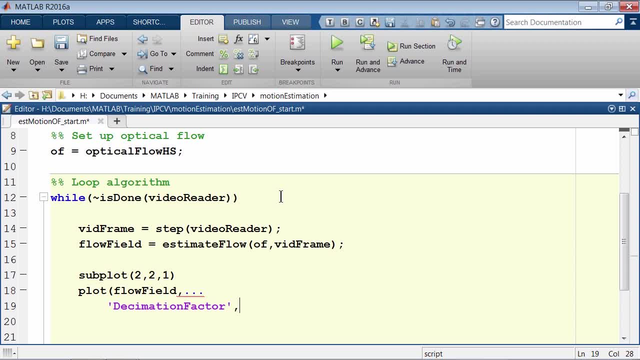 so that we can obtain a less cluttered plot. By default, this is a 1 by 2 vector 1, 1.. We can increase this to 10, 10 to get a less cluttered plot. Scale factor controls the length of the displayed vectors. 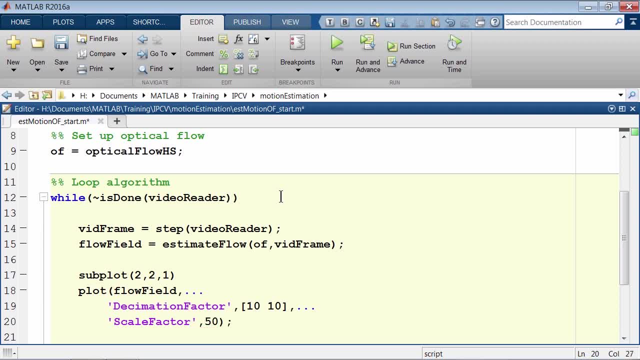 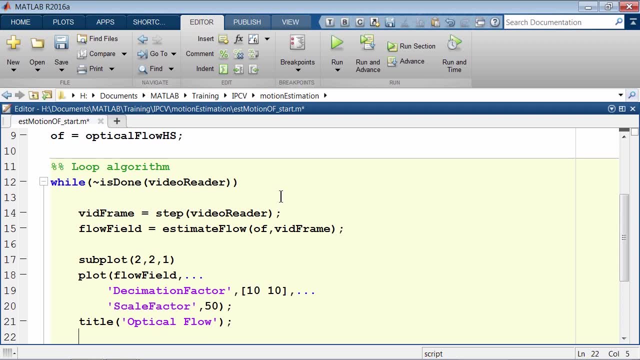 By default, this is 1.. We can increase this to 50 to see longer vectors. After this, let's set an appropriate title and then use the Draw Now command to update our figure instantaneously. for our iterations, Let's run this code. 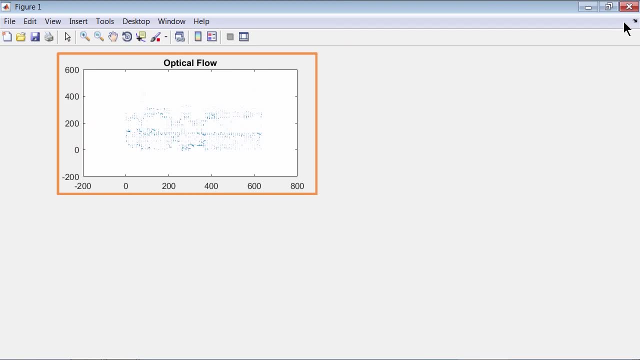 We see the quivers or arrows appear on our plot showing the motion field. If it was a single object moving against a static background, we would be able to get a sense for what kind of motion is depicted by our video frames. In our example, however, the entire scene is moving. 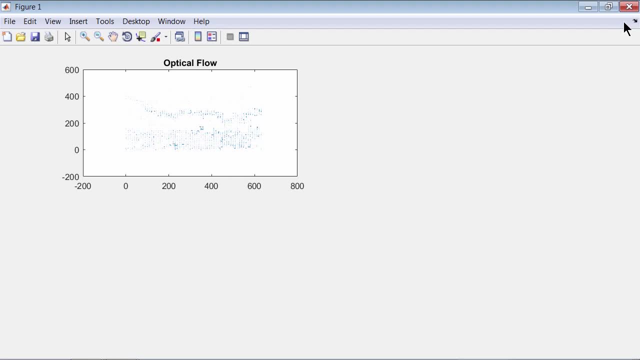 So it is more challenging to see the motion, to see from the motion field. what kind of motion is depicted in the video frames? Let's zoom in to the figure. We see the quivers that represent the motion field. Let's go back to MATLAB. 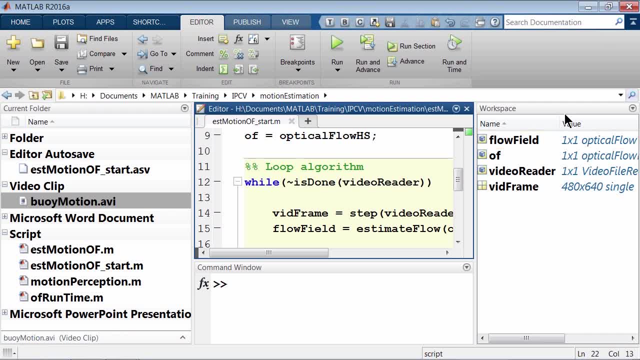 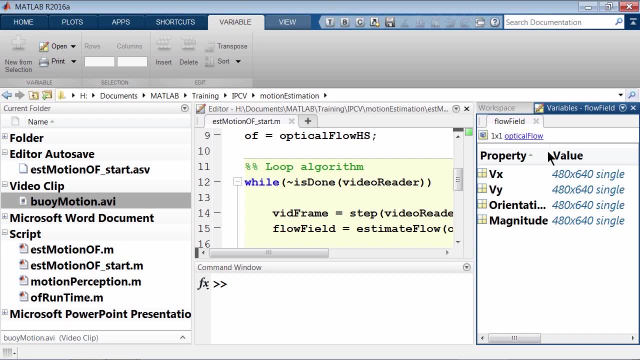 Here we see that flow field is an optical flow object. Let's double click on it to explore it. This contains information for all the pixels in the frame properties, such as the velocities in the x and y direction, orientation and magnitude. that has been represented in the figure that we just saw. 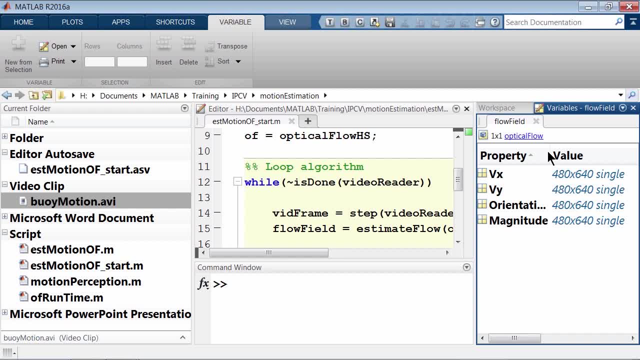 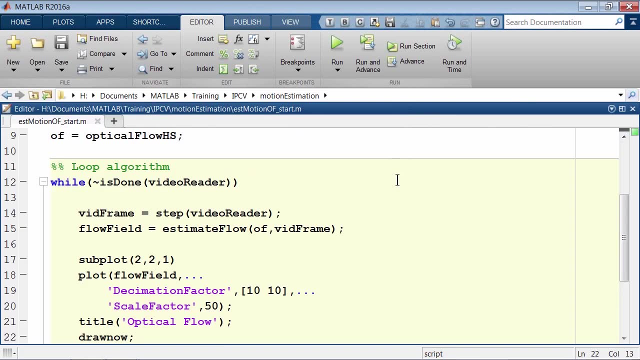 The velocities in the x and y direction are measured in pixels per frame. Recall that our final goal is to determine if the boat is moving towards the right or the left. To do this, let's go back to our script To determine if the boat is moving towards the right. 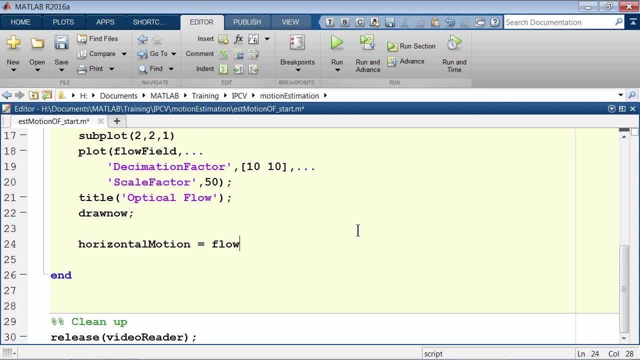 or left. we need only the velocity component in the x or the horizontal direction. We can then compare this to an upper threshold to look at only a subset of vectors that are greater than this threshold value to determine the objects moving to the right side. 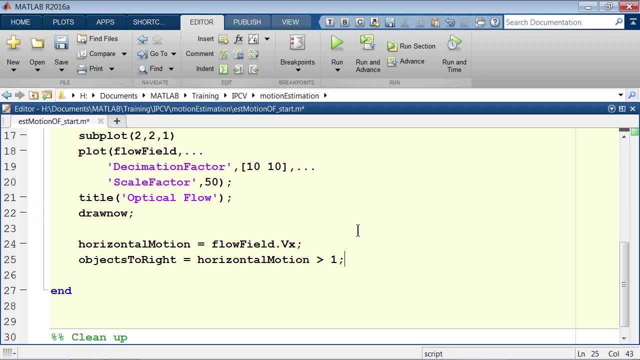 So by setting this threshold to a value of 1, we are computing all the pixels that have moved towards the right side, So we can see that the boat is moving towards the right by one pixel between frames. Similarly, we can compare this to a lower threshold. 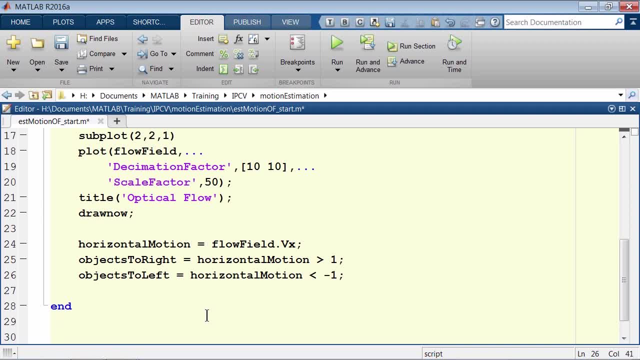 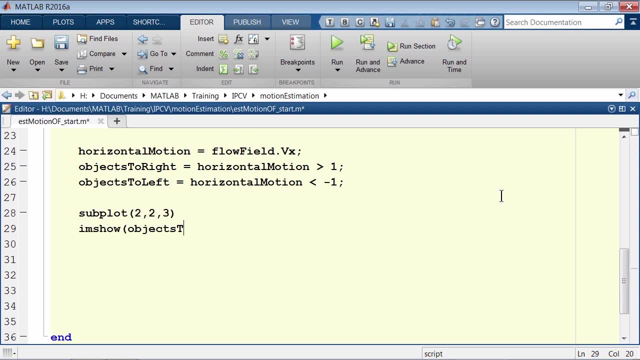 to look at only a subset of vectors that are lower than this value to determine the objects moving to the left side. The resulting logical matrices are just black and white images which can be viewed using IAMSHOW. Let's also set an appropriate title to these images. 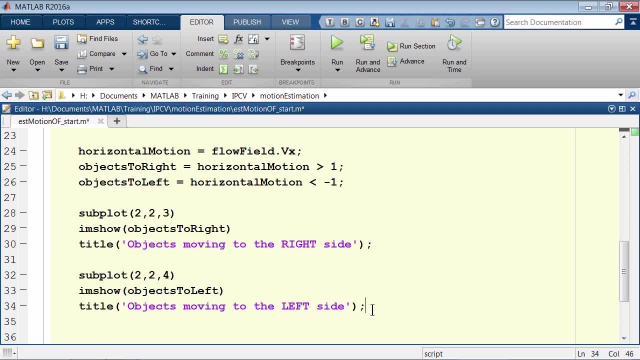 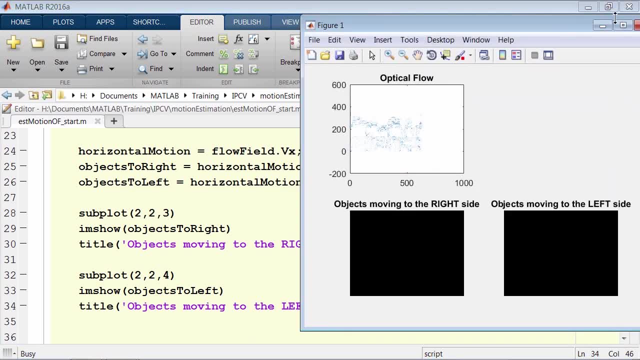 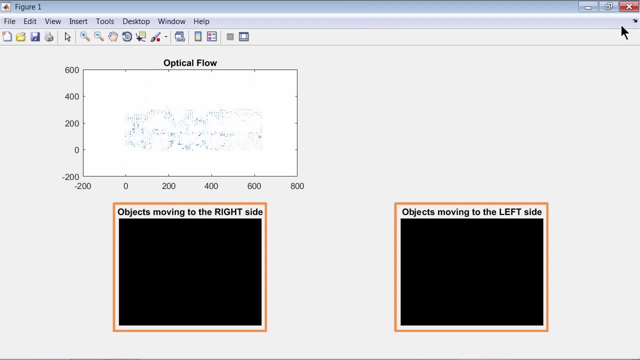 Let's run this code. We see only black images here. We are supposed to see the objects moving to the right or left. We are unable to see this because we have not properly tuned our optical flow algorithm, For example. in this case, let's go back to the script. 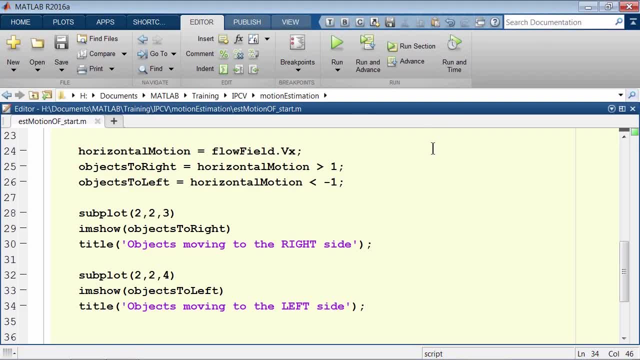 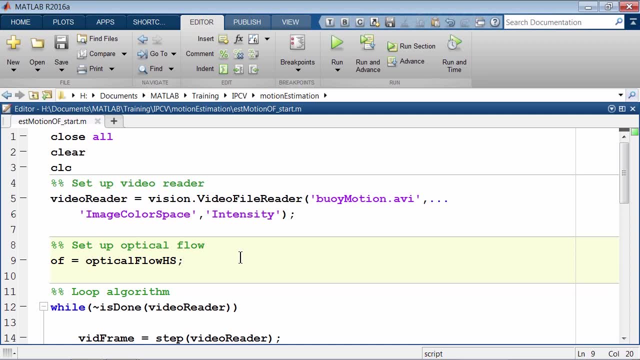 Let's run this code. Let's run this code. Let's go back to the script. We are using the Honshung method here. This algorithm has a smoothness property that can be tuned. Let's access this using the dot operator. 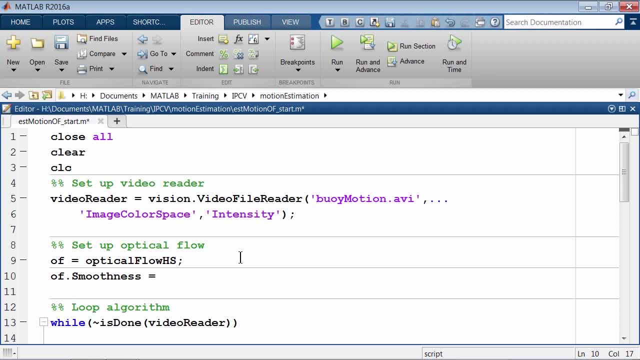 This is set to a value of 1 by default. We can increase this to detect larger movements. In our case, the video looks fairly smooth, so let's decrease it to detect smaller or smoother movements. So let's set it to a value of 0.1. 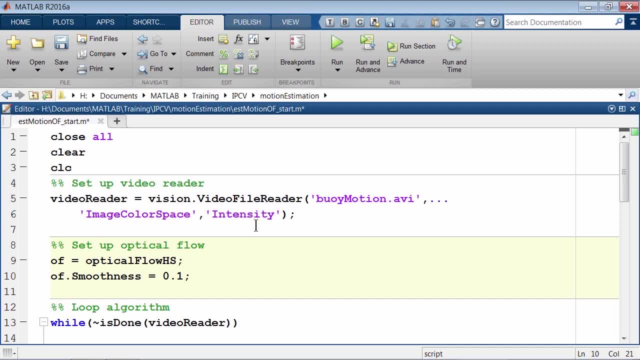 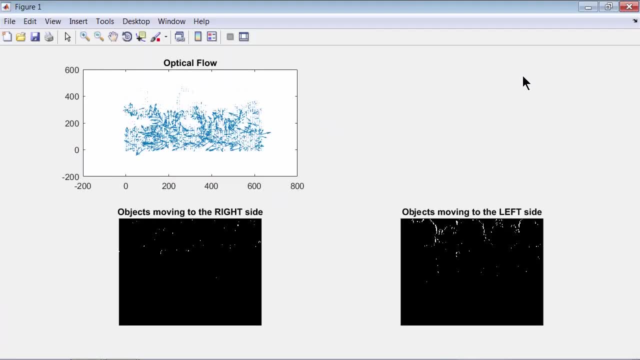 Let's run this code. Now we can see the two new black and white images. The image here highlights the objects moving towards the left, And the image here highlights the objects moving towards the right. With this information, we can determine if our robot is moving to the right or left. 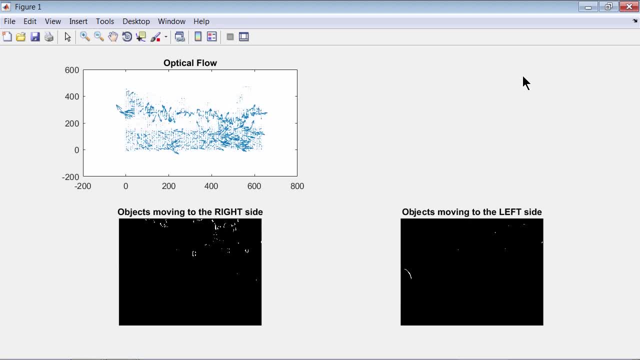 Let's run this code. Let's run this code. Let's run this code. If we detect more pixels moving towards the left. If we detect more white pixels moving towards the left, it updates this set. This checkbox also detects more pixels moving towards the right. 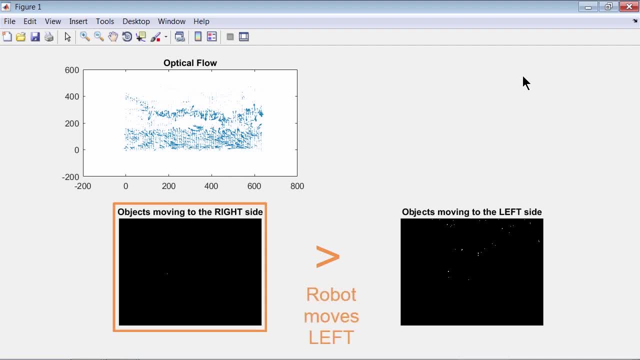 like this, Or in other words, if we detect more white pixels moving towards the left, لف or left- by counting the number of white pixels in each of these images. Our white pixels are the number of non-zero elements in our black and white images. 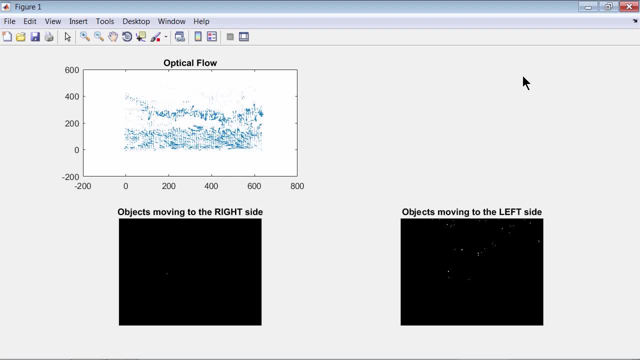 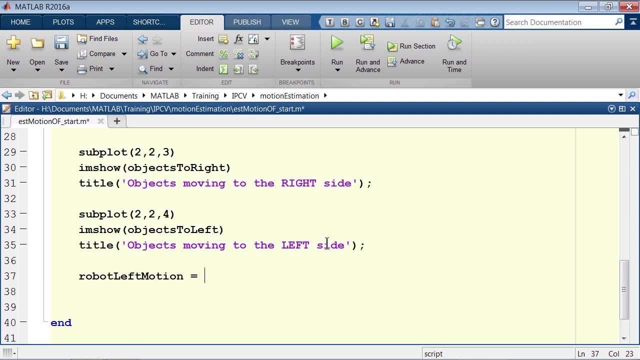 To compute this we can use the NNZ function. Let's go back to our script. So for left motion, we compute the number of non-zero elements in the objects to right image, And for the right motion, we compute the number of non-zero elements in the objects to left image. 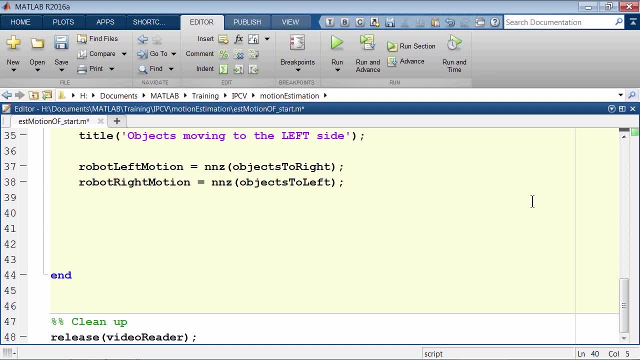 To determine if our robot is moving to the left or right. we can do a comparison between the two white pixel counts. If the robot left motion is greater than the robot right motion, we can set a string to a value moving to left. Else, we can set the string to a value moving to right. 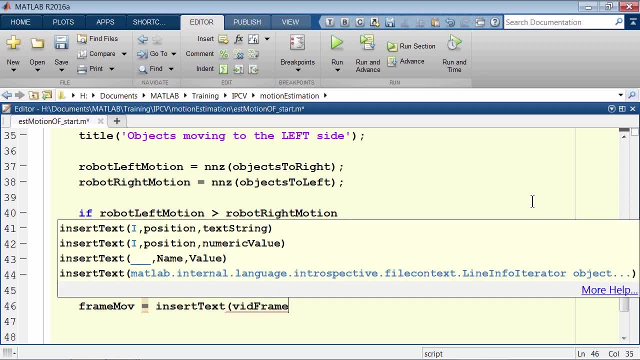 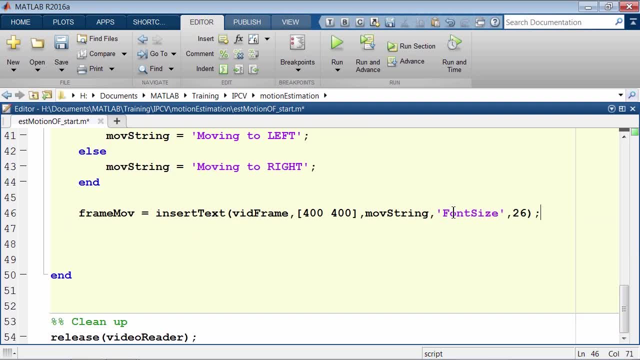 Using this, we can visualize the robot as moving to the left or to the right. We can also see the result by inserting the text on our video frame at a fixed location and a large font, and then display it using, I am sure. 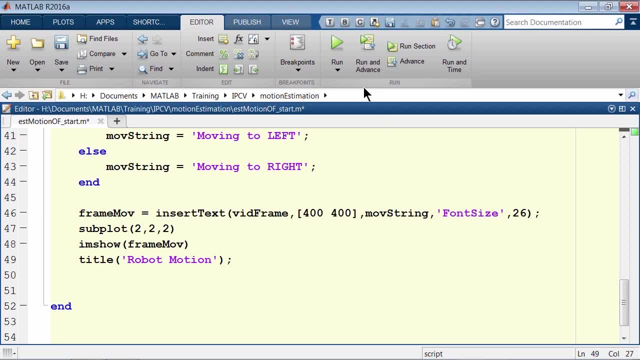 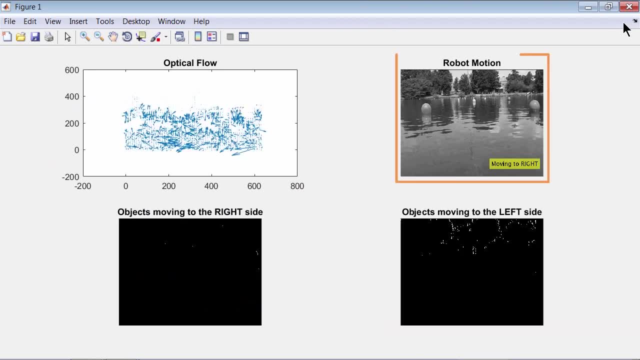 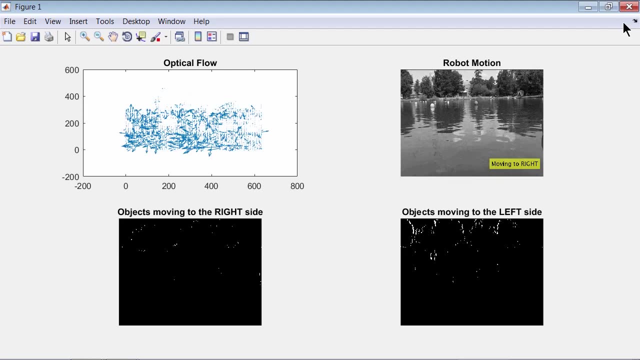 Let's set an appropriate title for this image as well. Let's run the script. Now we see the video and the text showing us the result. Let's run the script. Let's see the direction of motion When we compare the black and white images. 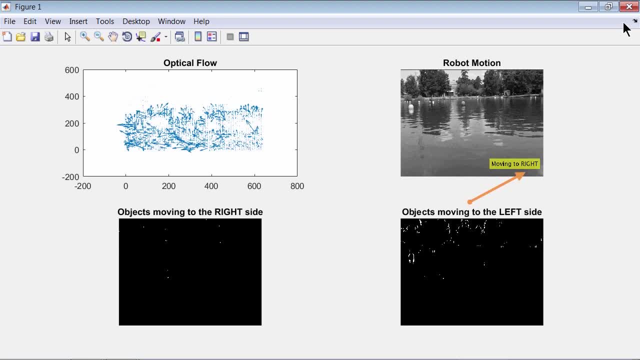 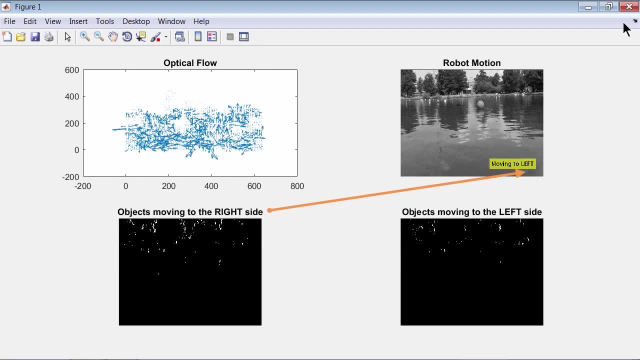 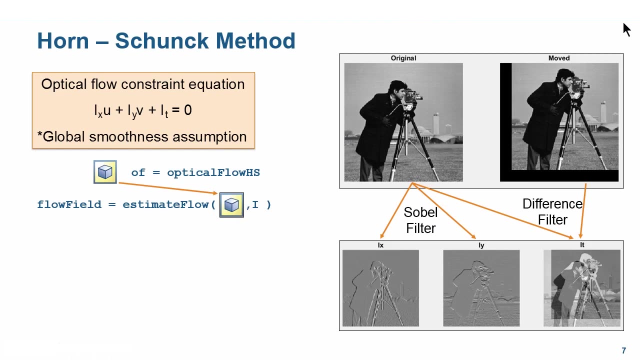 we can see that whenever there are more white pixels in this image, the robot is moving towards the right. Whenever there are more pixels in this image, the robot is moving towards the left. Let's go back to the presentation. We talked about the Horn-Schrank method. 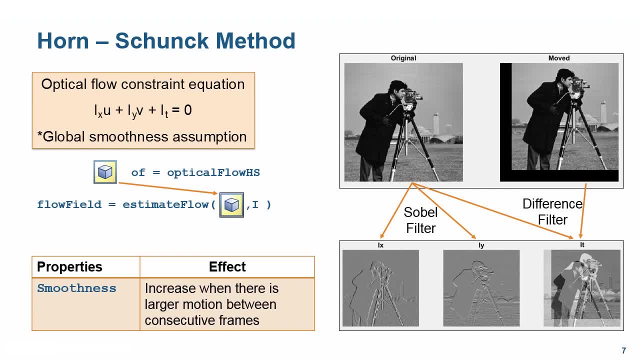 We discussed the smoothness parameter. Please refer to the documentation link in the resources section to get a full list of parameters supported for this algorithm. In our example, we decreased it to detect smoother movements. We can increase this to detect larger motion between consecutive frames, but this also 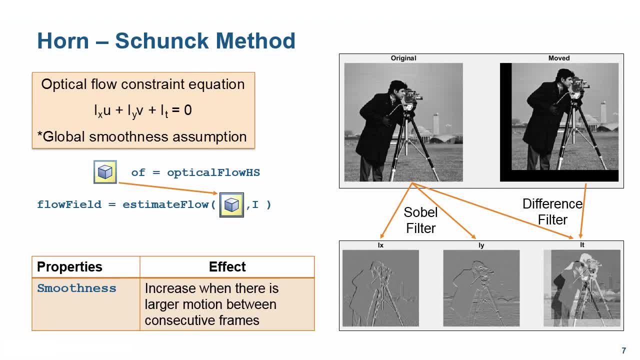 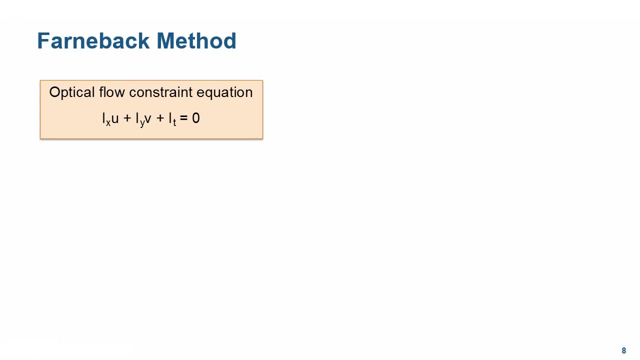 slows down the computation because now the search space is bigger. If we expect the displacement of pixels between the consecutive frames to be large, we can use the Farnbach method instead. The Farnbach method also solves for the optical flow constraint equation. 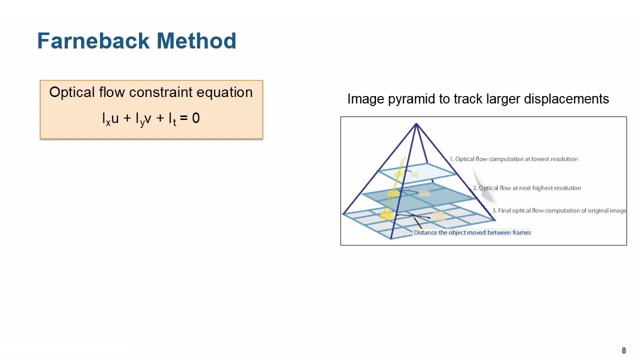 It does this by constructing an image pyramid with n levels, where n can be specified by the user. Each level has a lower resolution compared to the previous level. The algorithm can track points at multiple levels of resolution, starting at the lowest level. Increasing the number of pyramid levels enables the algorithm to handle larger displacements. 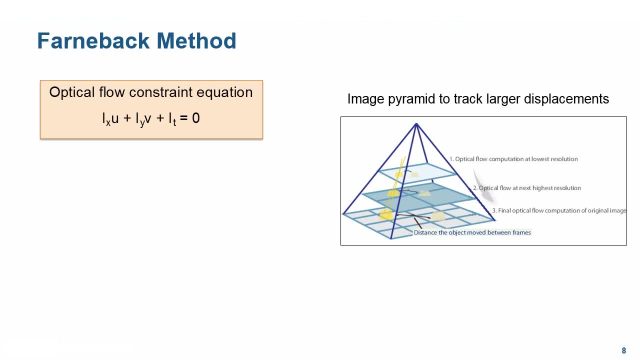 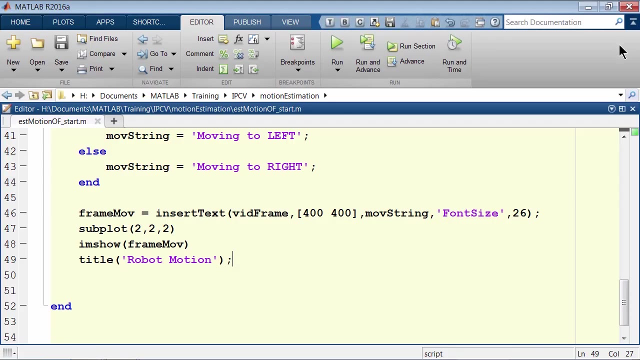 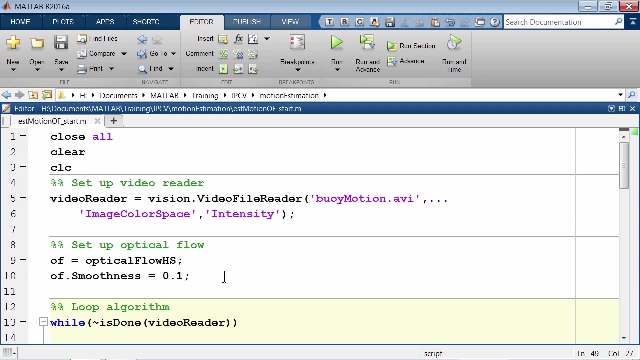 of points between frames, However, the number of computations also increases. We can implement this in the Computer Vision System toolbox using the optical flow Farnbach object. Let's switch to MATLAB to see how we can do this In the script we developed. let's go back to setting up the optical flow. 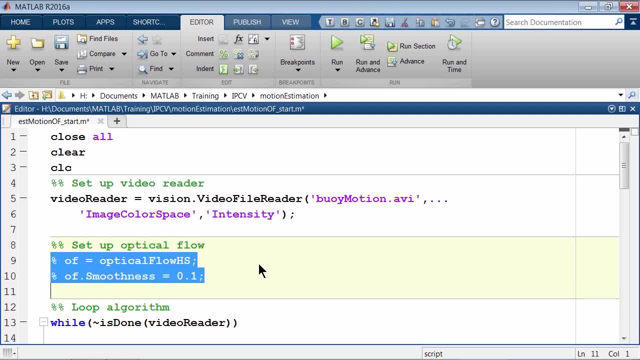 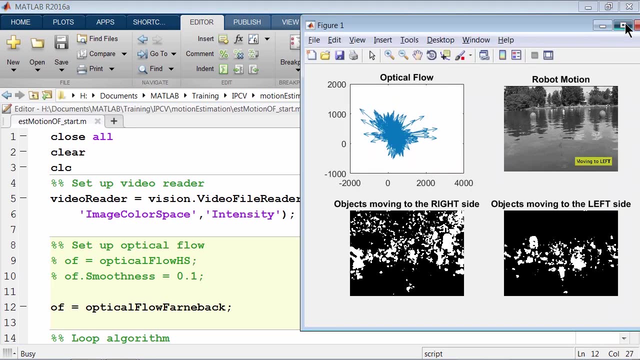 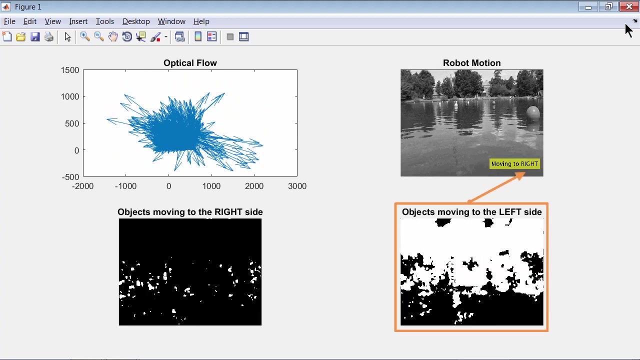 Comment the code for the Horn-Chunk method. Instead we will create the object using the Farnbach algorithm with the optical flow Farnbach object. Let's run the script. We can see the motion estimation. The boat is moving to the right first. 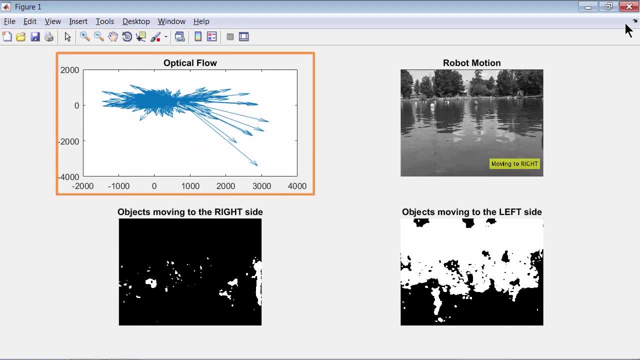 Notice also the denser field. as a result of the Farnbach The boat is moving to the right first Notice also the denser field. as a result of the Farnbach The boat is moving to the left first Notice also the denser field. as a result of the Farnbach. 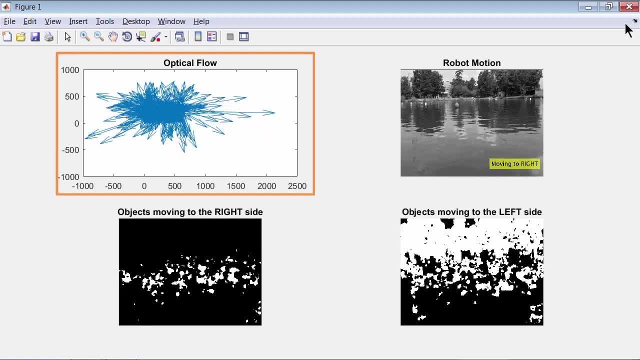 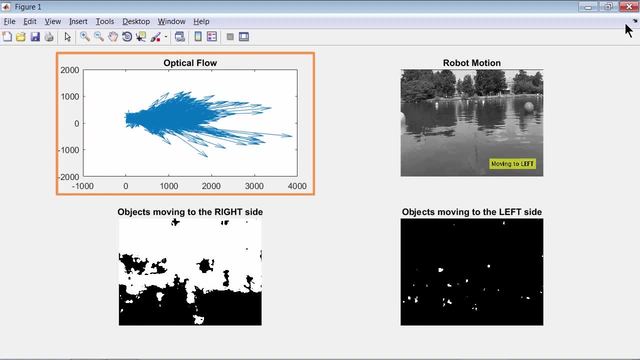 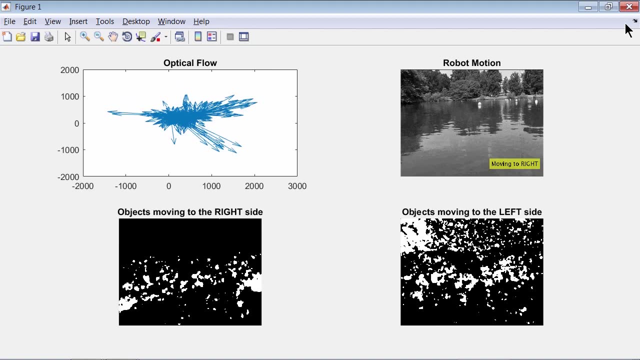 Notice also the denser field. as a result of the Farnbach, It is best suited to detect large displacements. so even the smooth, smaller movements between our video frames result in an amplified optical flow field. The algorithm by default uses 3 levels of pyramid that we just discussed. 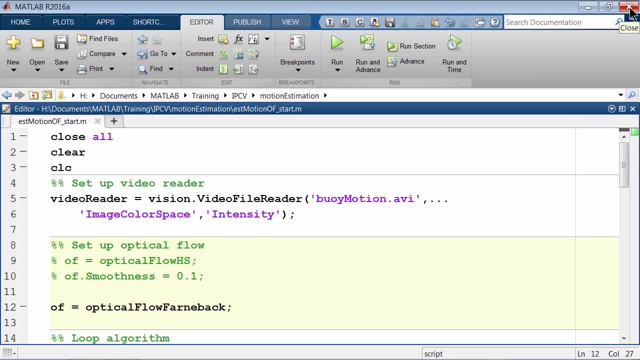 This can be changed, so let's go back to our script. Let's use the dot notation again to set the number of pyramid levels. using the numPyramidLevels property, We can increase this to detect larger displacements. In our case, the displacements are not that large, so let's set the pyramid level to 1.. 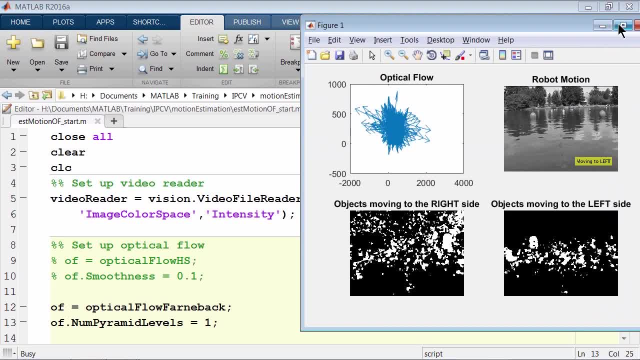 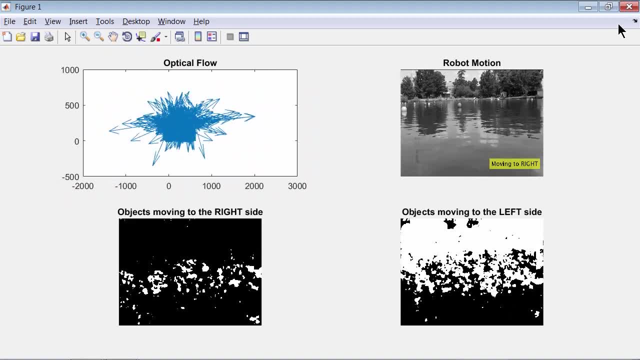 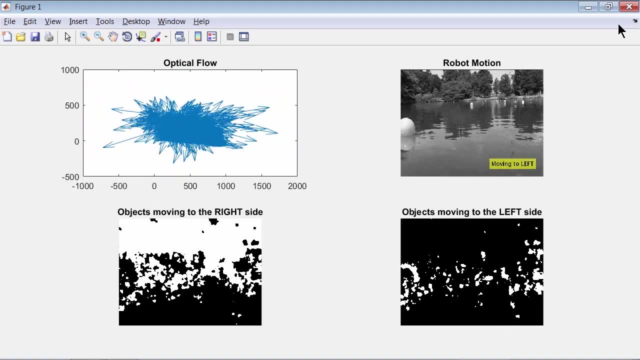 Let's run the code again. It looks like we haven't lost the dense fields. This is good because for lesser pyramid levels we are obtaining similar results, which means we can set it to a smaller number to get a better performance. Let's go back to the presentation. 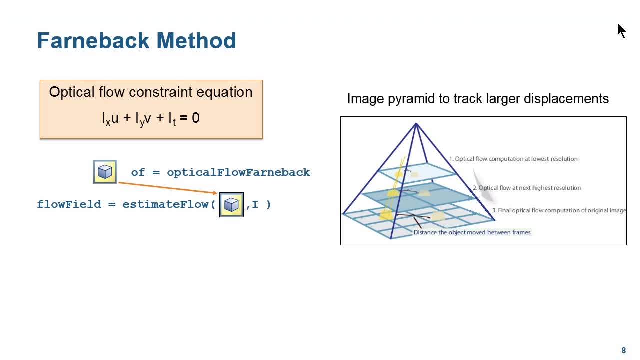 We just talked about the fanback algorithm. It uses pyramid levels to track larger displacements. This can be controlled using the numPyramidLevels property. Note also that the algorithm has a filter size property that can be increased to make the algorithm more robust to noise. 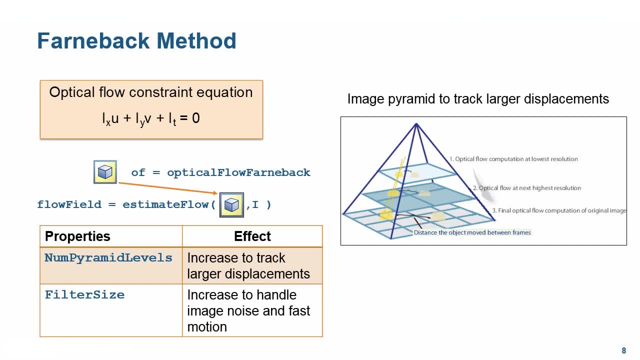 Please refer to the document. There is a presentation link in the resources section to get a full list of parameters for this algorithm. Recall that fanback is also a dense flow algorithm, which means it also processes the entire image, leading to accurate fields, but higher computation time. 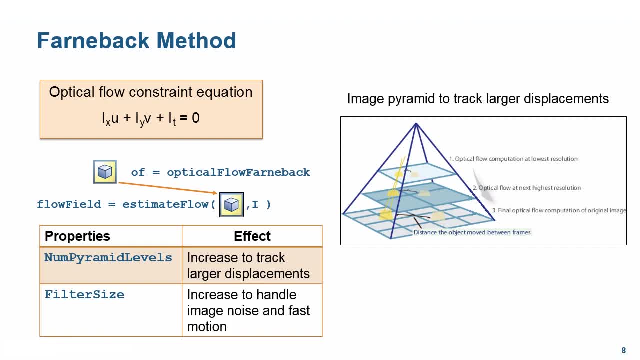 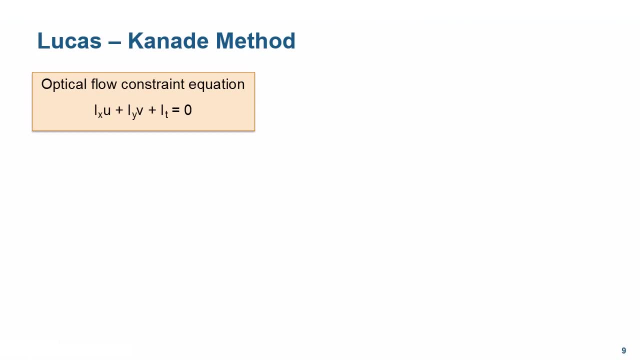 The other kind of optical flow method is the sparse flow method. Lucas-Canary is a sparse flow method that also solves for the optical flow constraint equation If we have two image frames. the Lucas-Canary method uses a custom filter to calculate the 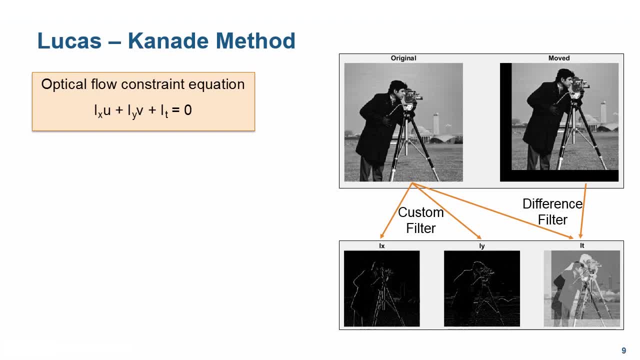 spatial gradients and a difference filter to compute the temporal gradient. After this, the method divides the results into smaller sections to obtain the optical flow vectors. Since it operates only on sections of images, this results in faster computations, although sometimes this could lead to less accurate results. 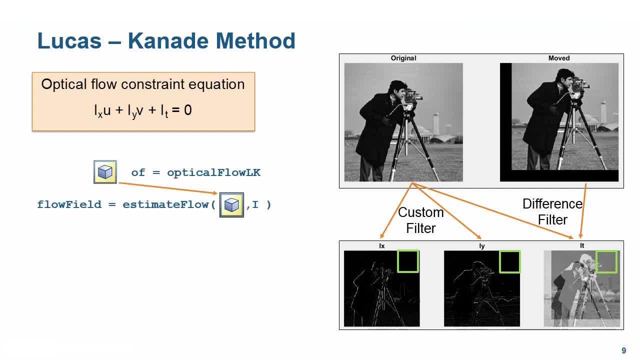 We can implement this in the computer vision system. We can also use this method to calculate the spatial gradients. If we have two image frames, the Lucas-Canary method uses a custom filter to calculate the spatial gradients, And if we have 3 image frames, the Lucas-Canary method uses a custom filter to calculate the. 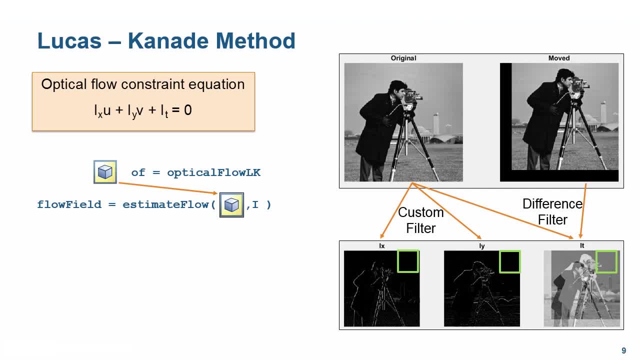 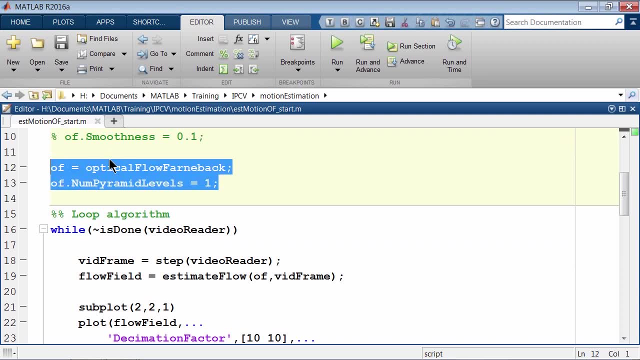 spatial gradients And if we have four image frames, we can use this method to calculate the spatial gradients of each image frame. Let's switch to MATLAB to see how we can do this In the script we develop. let's comment the optical flow by the fanback method. 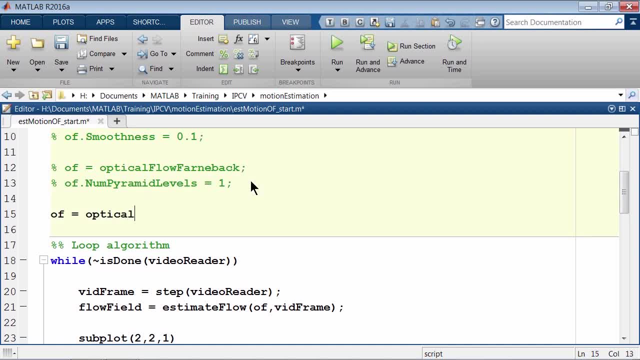 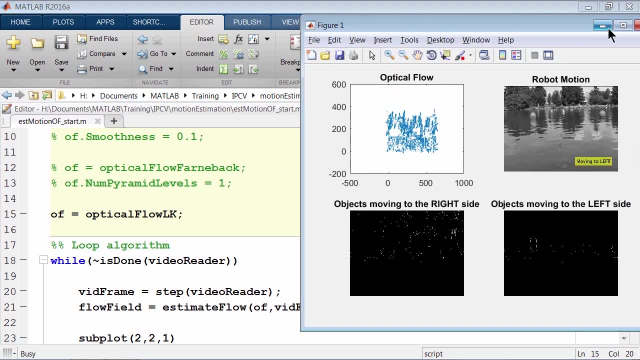 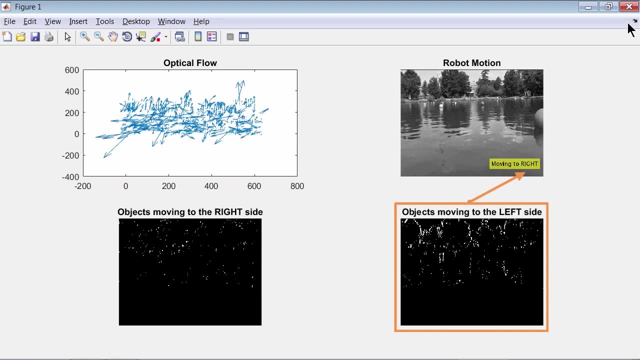 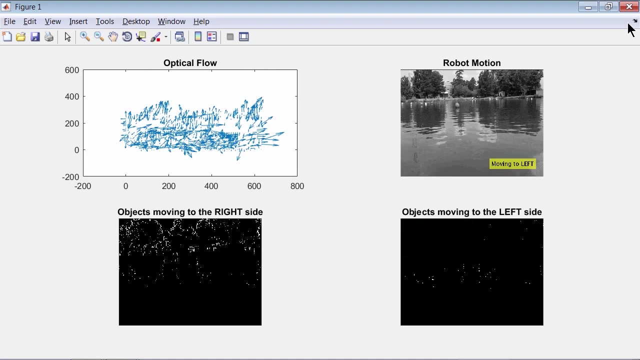 Instead, we will create the object using the Lucas-Canary algorithm with optical flow: lk object. Let's run the script. We can see the motion estimation Boat is moving to the right first. Notice the detected tree line. If we record the runtime of this code using tick-tock commands, 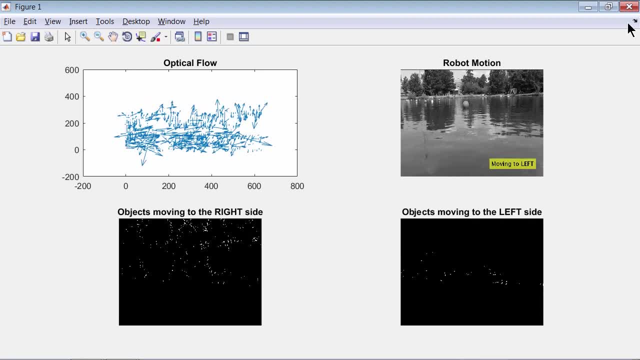 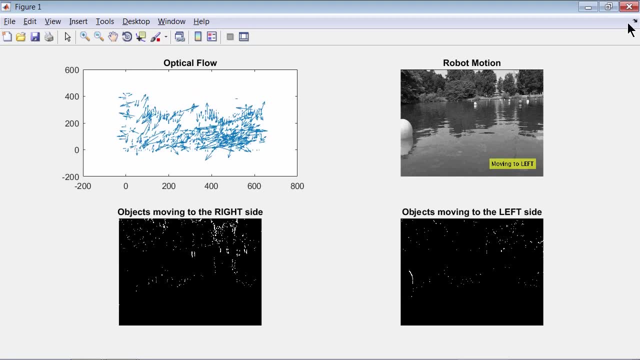 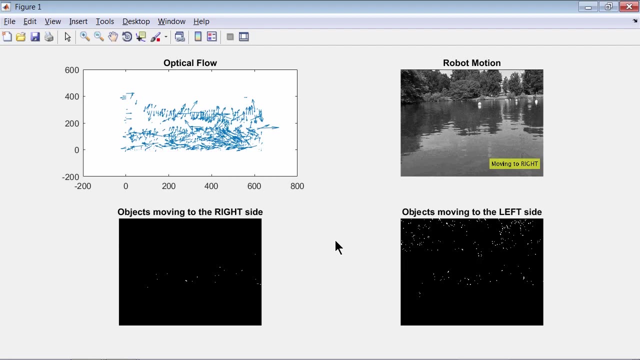 we can see that this method performs faster compared to both the dense flow methods, namely the haunt shunk and farm back. Refer to the provided MATLAB code file, opticalflow-runtimem, to compare the runtimes of the different algorithms. Let's go back to the script. 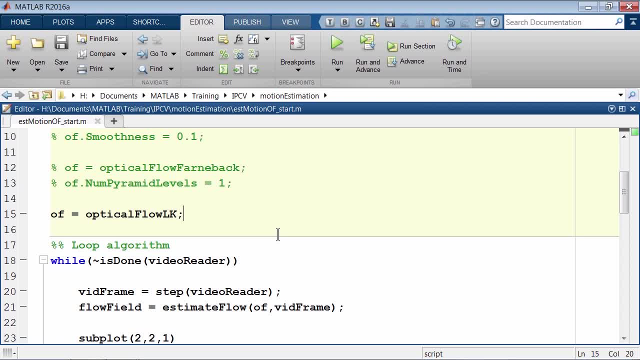 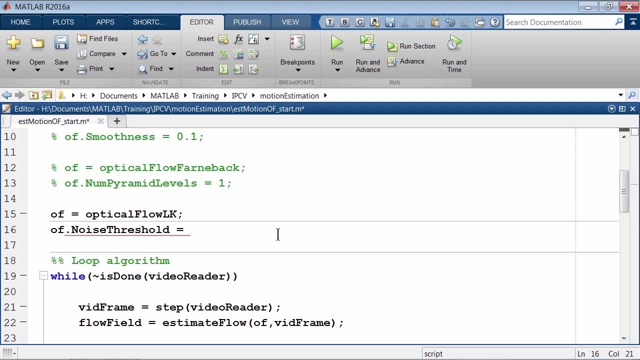 The only property we can tune for the Lucas-Canada method is the noise threshold. Let's access this using the dot notation. By increasing this, we can be more selective of the detected motion and potentially decrease the effect of noise. Note that higher values might result in the algorithm filtering out even valid motion. 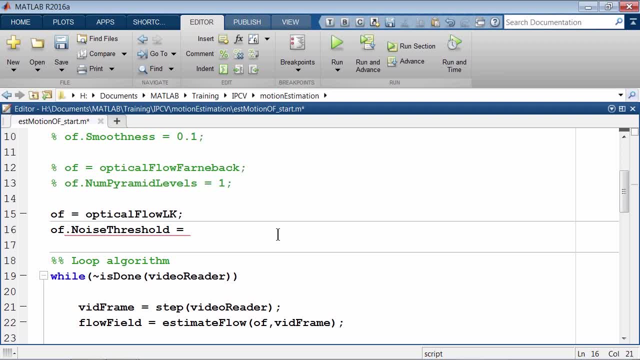 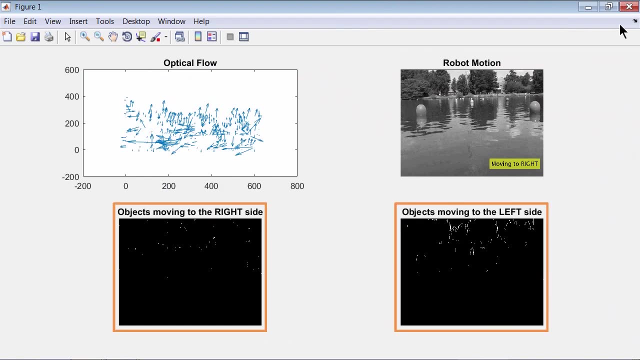 The default value is 0.0039.. In our case, let's set the noise threshold to a higher value: 0.01.. Let's run the code again. We can see the slightly thinner but more defined field. The noise seems reduced. 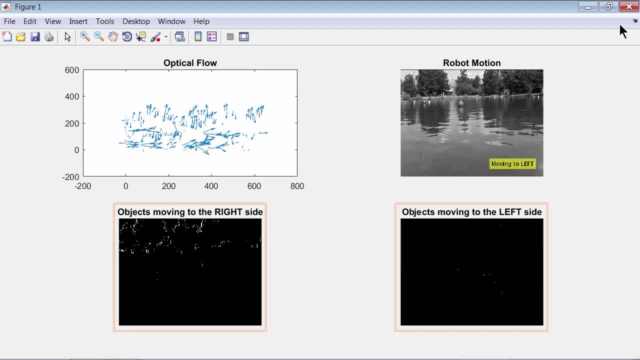 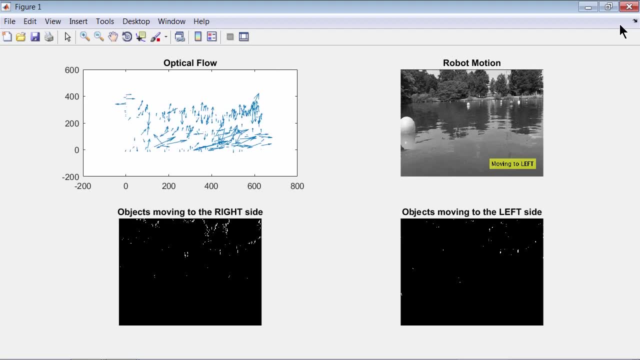 We can see less motion detected based on the movement of the water. The base Lucas-Canada method uses a difference filter for the temporal gradient, which is simple and hence results in faster results. The high side performance, Api, in your case, is lower than normal. 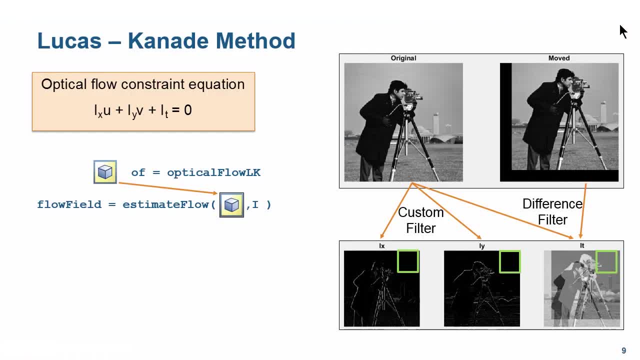 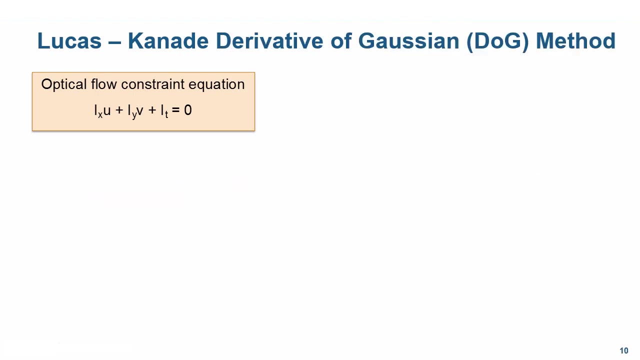 but the animation output is only 1,040.. So you can jump past the total of 1,040 to find out for the current one. If you look into theArtcom page in the sidebar a chart of subtitles is drawn. 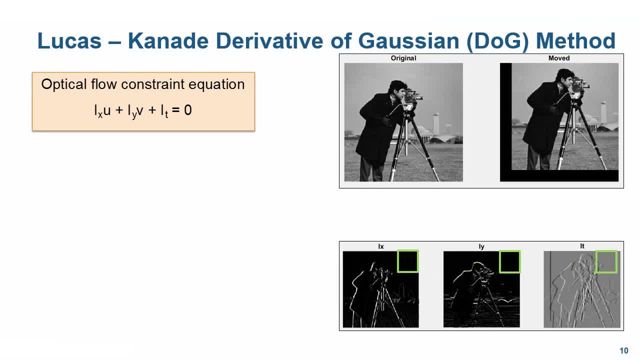 It can't be stopped. The bottled 可以 be shown on the white things that it solves for the optical flow constraint equation in sections. It is different in the nature that it uses different filters to compute the spatial and temporal gradients. It uses a Gaussian and a derivative of Gaussian filter. 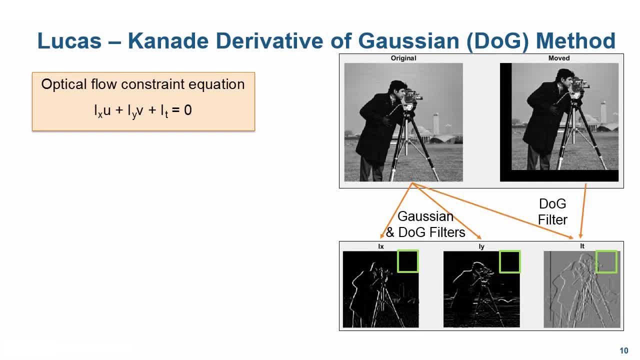 to compute the spatial derivatives and a derivative of Gaussian filter to compute the temporal derivative. This leads to operating the base Lucas-Canady method with better noise rejection. This can be implemented in the computer vision system toolbox using the optical flow LKDOG object. 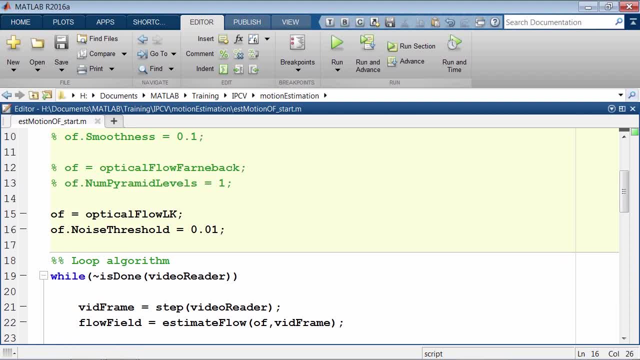 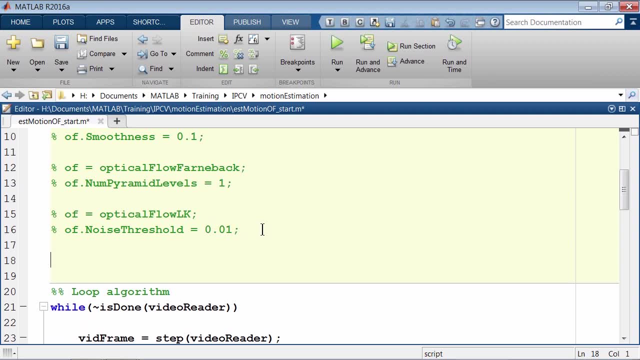 Let's switch to MATLAB to see how this works In the script we developed. let's comment the optical flow by Lucas-Canady method. Instead, we will create the object using the Lucas-Canady derivative of Gaussian algorithm with the optical flow: LKDOG object. 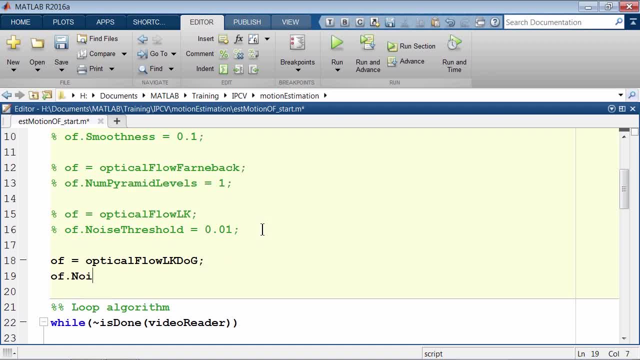 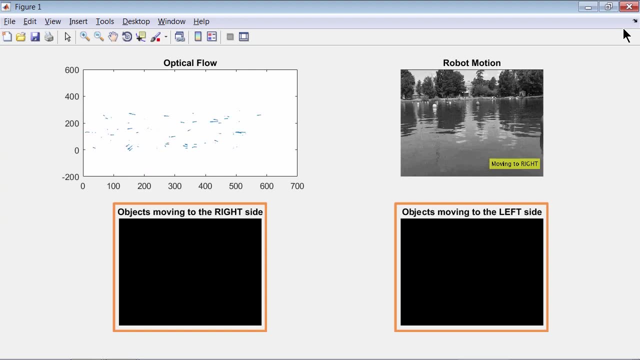 This algorithm also has a noise threshold property and let's set it to the same value as the base Lucas-Canady method. Let's run the script. We only see black images here. This is because the Lucas-Canady derivative of Gaussian method. 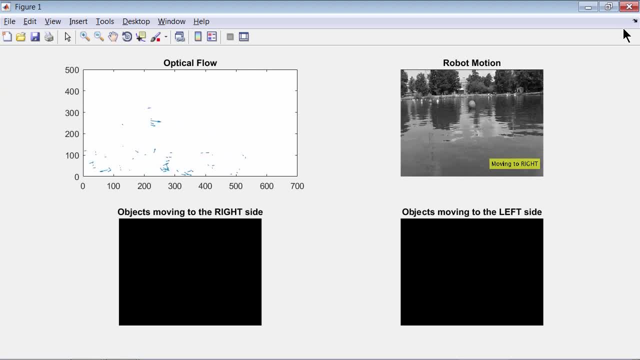 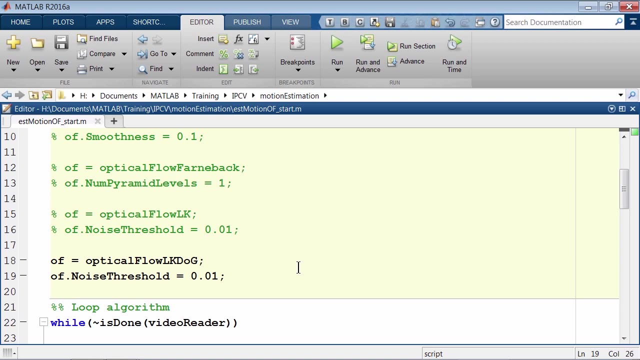 lets us operate on the Lucas-Canady method with a smaller noise threshold because of more configurable filters in the algorithm. Let's go back to the script. The default value for the noise threshold is 0.0039.. In our case, let's set the noise threshold to something smaller. 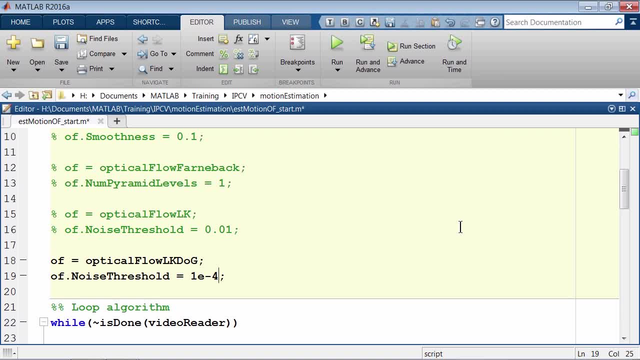 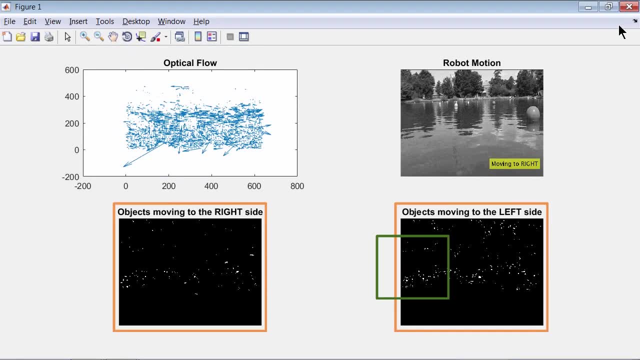 Let's say 1e minus 4.. Let's run the code again. We can see the slightly thinner tree line. We can also see the buoys. We can see that the boat is first in line. We can also see the buoys. 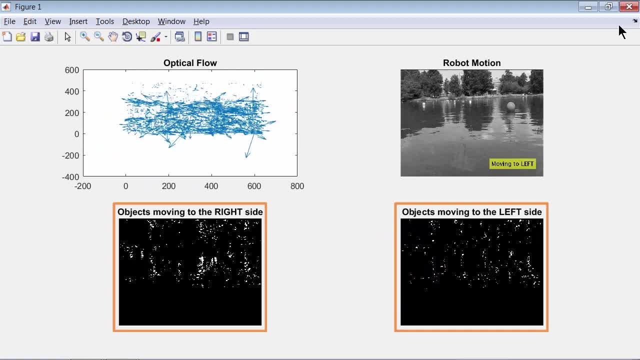 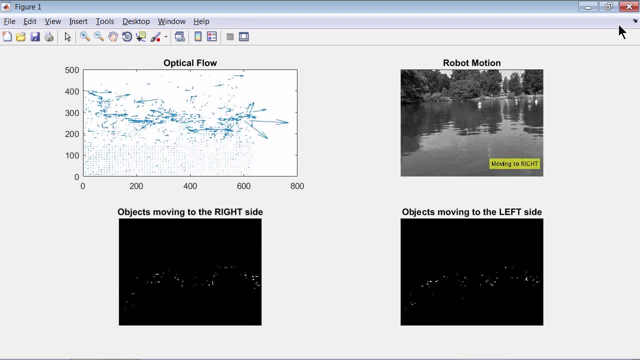 We can see that the boat is first in line. We can see that the boat is first in line And the boat is first moving towards the right And then it is moving towards the left. Note that we have not talked about all the properties. 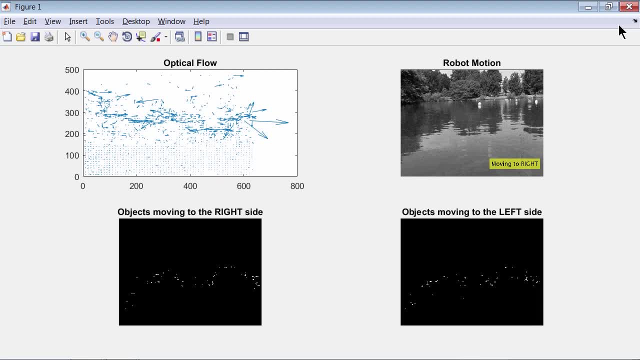 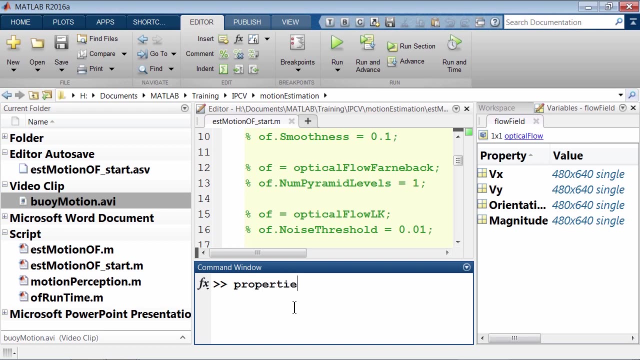 applicable for each of the algorithms discussed here. We can use the properties command on any of these objects to get a full list of all the properties supported by the algorithm. Let's go back to the command prompt here. So here we can say: properties of our optical flow object. 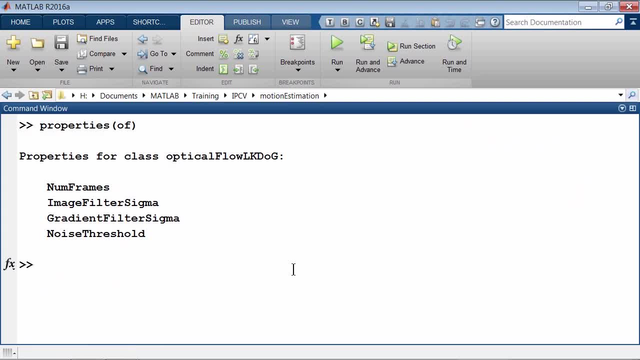 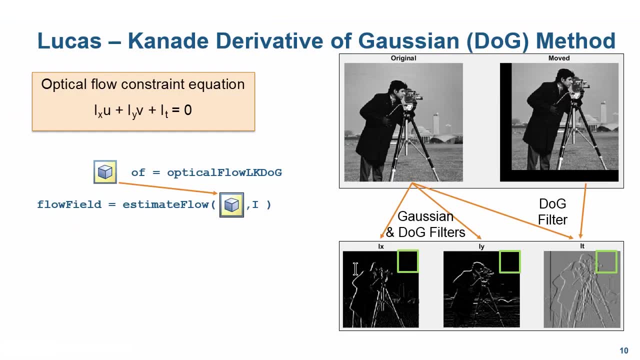 to see all the properties associated with this particular algorithm. Let's go back to the presentation. We talked about the Lucas-Canady derivative of Gaussian method. We talked about the noise threshold property, similar to the base Lucas-Canady method, which can be increased to reduce noise effects. 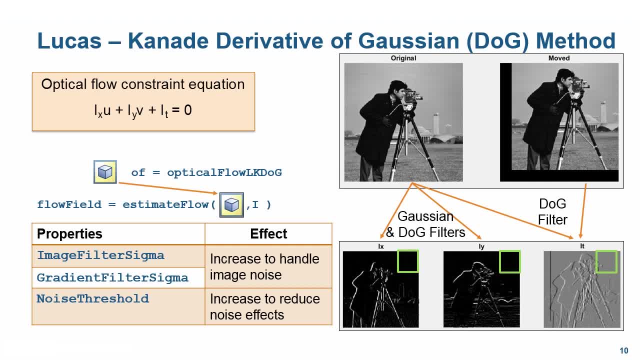 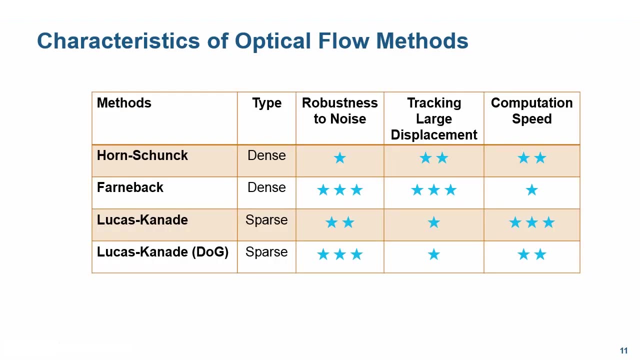 The filters in this method can be configured using the image filter sigma and the gradient filter sigma parameters. This makes the algorithm more robust to noise. It also lets us operate on the base Lucas-Canady method with a reduced noise threshold. In summary, we talked about four different optical flow methods. 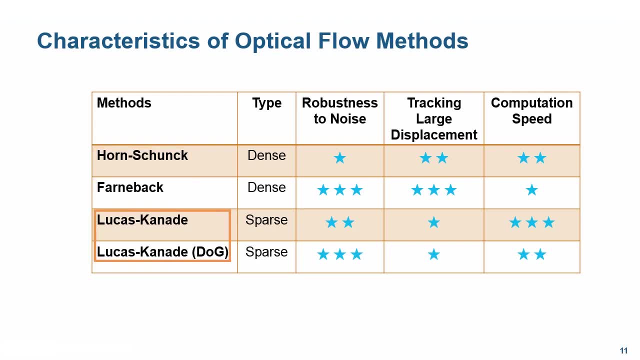 Horned, shunk and fawn back are the dense methods and the two variations of the Lucas-Canady method are sparse methods. Fawn back and the Lucas-Canady derivative of Gaussian method have the ability to change the frame rate of the image.